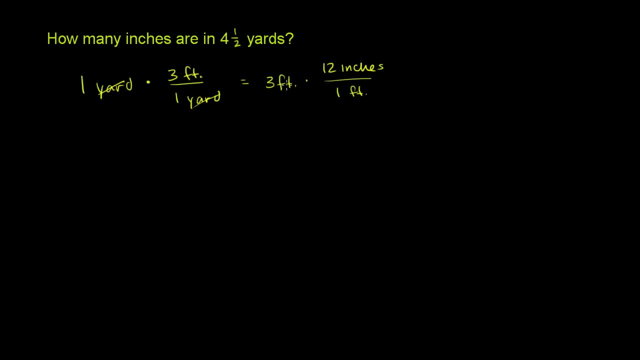 3 feet is going to be more inches. We're multiplying by 12. And also these units cancel out Foot in the numerator, foot in the denominator. 3 times 12, divided by 1, is equal to 36 inches. 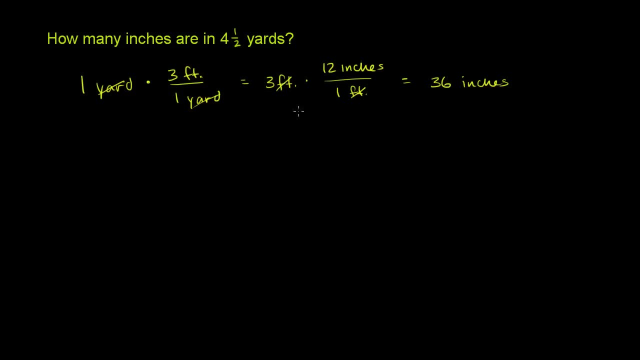 So you might have already known it, but this is nice to have the dimensions cancel out like this. We know that 1 yard is equal to 36. 36 inches, Or there are 36 inches for every 1 yard, And so we can now either break this down. 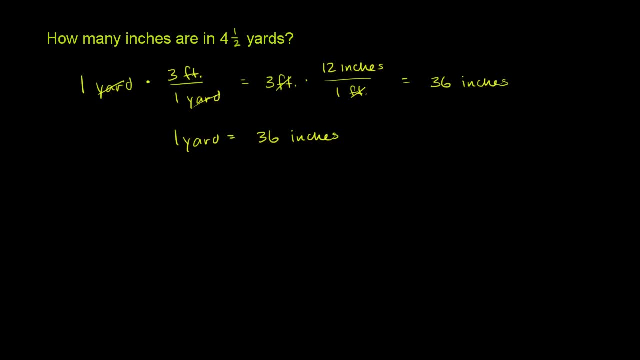 or we could turn this into an improper fraction. First I'll just break it down into 4 yards plus 1 half yards, So we could say that this is 4 yards. So 4 yards is going to be equal to well. 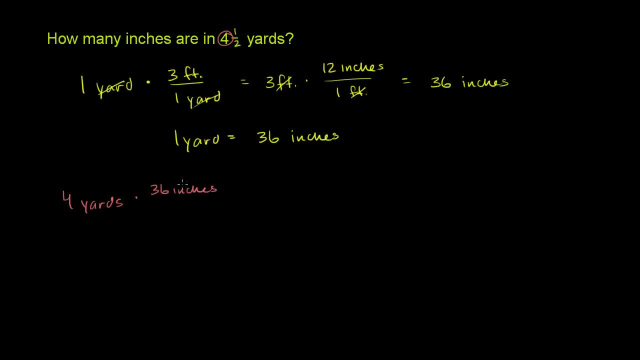 let's just multiply it times 36 inches for every 1 yard The yards cancel out. 4 times 36 is 100.. 120 plus 24.. So that's 144.. So this is equal to 144 inches. That's just the 4 yards. 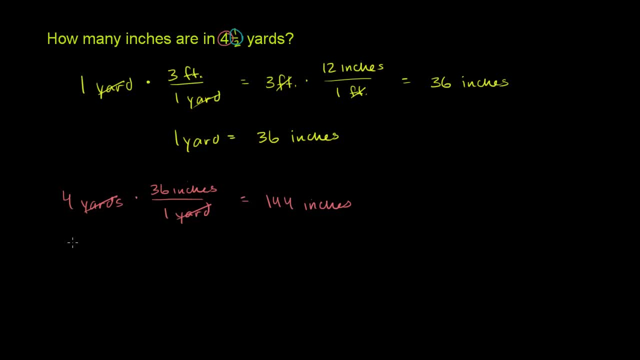 And then if we do the half yards, so 1 half of a- I guess I should say 1 half yard, once again times 36 inches per yard, The yards cancel out. 1 half times 36 is going to be equal to well. 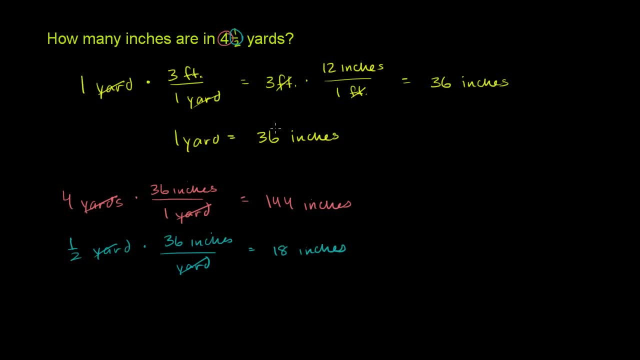 1 half. That's equal to 18 inches. So 4 and 1 half yards is the same thing as 4 yards plus 1 half yards, which is the same thing as 144 inches plus 18 inches, which is going to give us- let's just add it up over here- 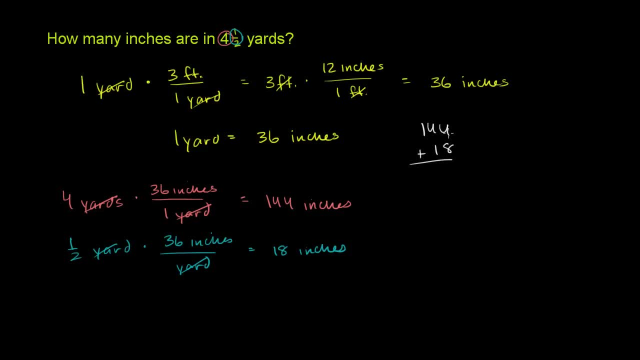 on the right: 144 plus 18.. 4 plus 8 is 12.. 4 plus 1 is 5.. You have this 1 up here, So it's 6. And then we have a 1. So when you add them all together, you get 162 inches. 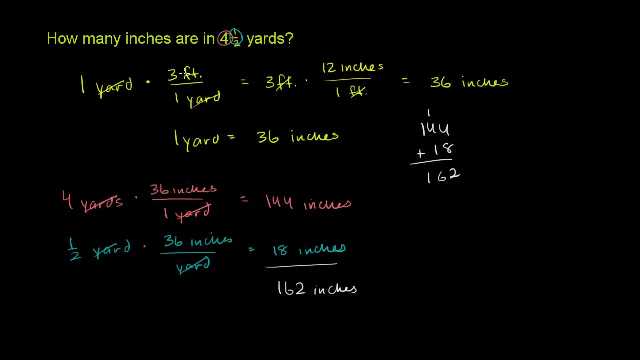 The other way to do this would have been to convert this into an improper fraction and then multiply by the units. So let's do it that way. If I have 4 and 1 half of anything really, so let me write 4 and 1 half trying. 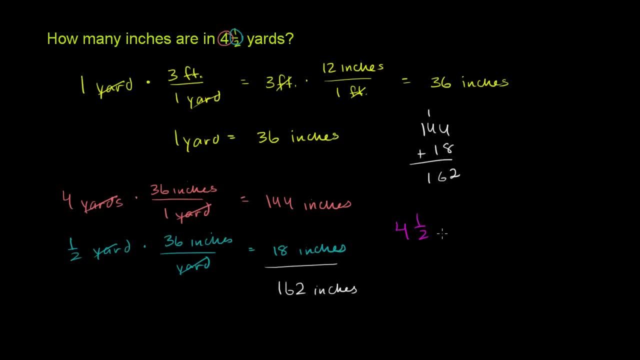 to find a suitable color. So if I have 4 and 1 half, this is the same thing. 4 is the same thing as 8 halves, This is the same thing. So let me write it this way: 4 and 1 half is the same thing as 4 plus 1 half, which. 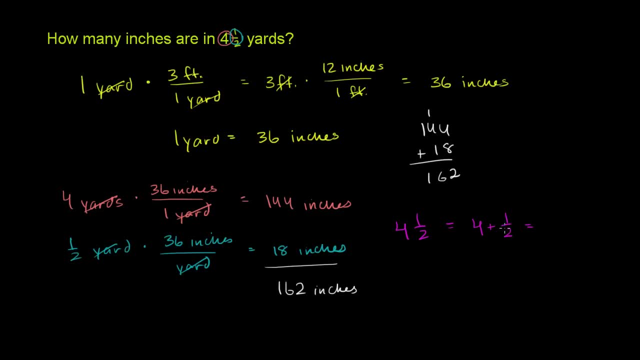 is the same thing as 4, if we want to have the same denominator as this- 2 over here, or is it this 1 half over here- This is the same thing as 8 over 2.. Or you could say 4 over 1 is the same thing as 8 over 2,. 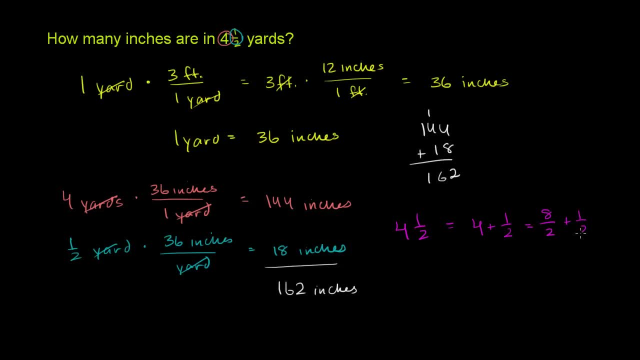 if we want to have a common denominator. So 8 over 2 plus 1 over 2.. Actually, let me write it that way, just so you really understand what we're doing. 4 is the same thing as 4 over 1.. 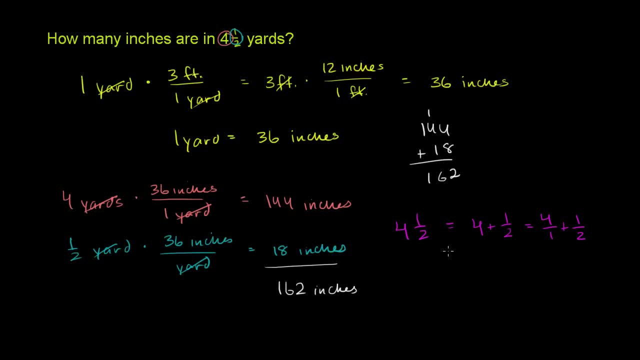 So it's 4 over 1 plus 1 half. If we want to find a common denominator, it's 2.. So 4 over 1 is the same thing as 8 over 2 plus 1 half, which is equal to 9 halves. 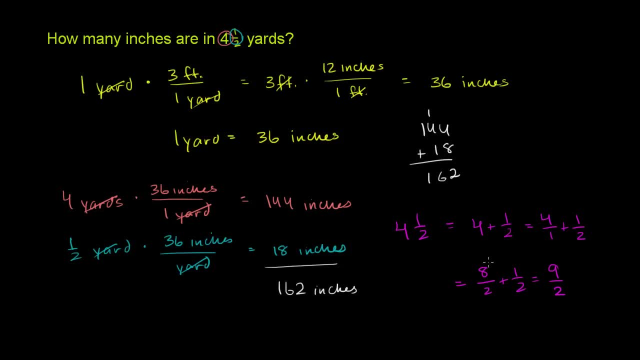 Now I did it this way, which takes longer, just so you really understand how we converted it, why it makes hopefully, conceptually, why it just makes intuitive sense, why 4 and 1 half is the same thing as 9 halves. 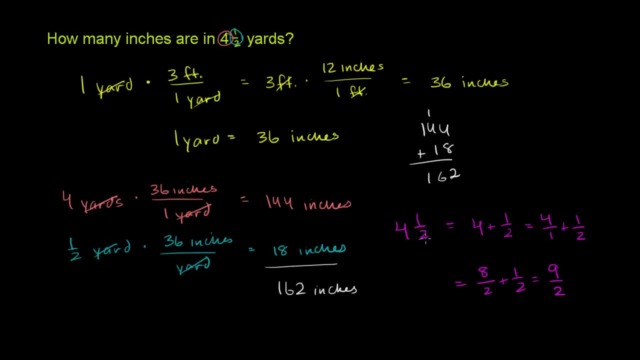 But if you want a simple process for it, you could just say: look, 4 times 2 is 8.. 8 plus 1 is 9. And that gives you that 9 right over there. so 9 halves. 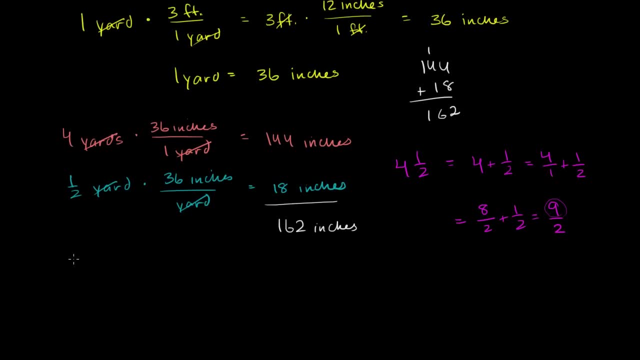 So we have 9 half yards that we want to convert to inches. So we have 9 half yards that we want to convert to inches. Same process Times 36: inches per yards. yard in the numerator, yard in the denominator, We are left with 9 over 2 times 36.. 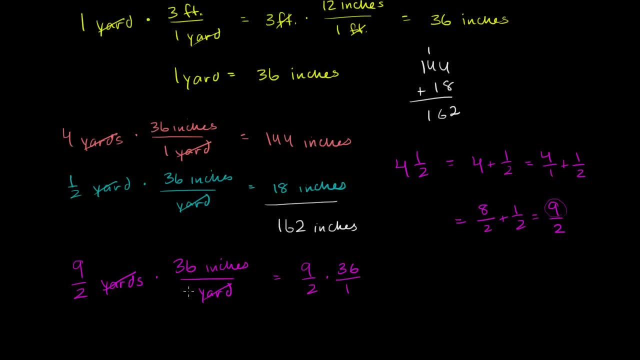 We could say times 36 over 1,, if we like, Times 36 over 1,, 36 inches for every 1 yard, Or the number 36 really is the same as 36 over 1.. And then we're left with just inches in our units. 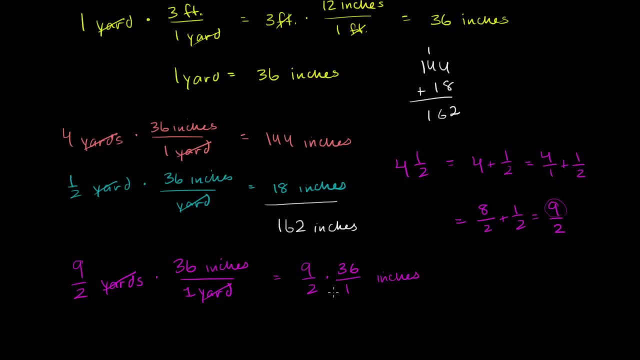 We're just left with inches And over here. there's several ways that we can simplify it. Probably the easiest way to simplify it is we can divide both our numerator and our denominator by 2. So let me write it this way. I don't want to skip steps.